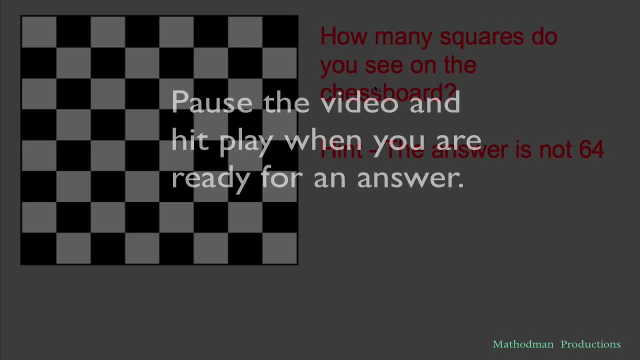 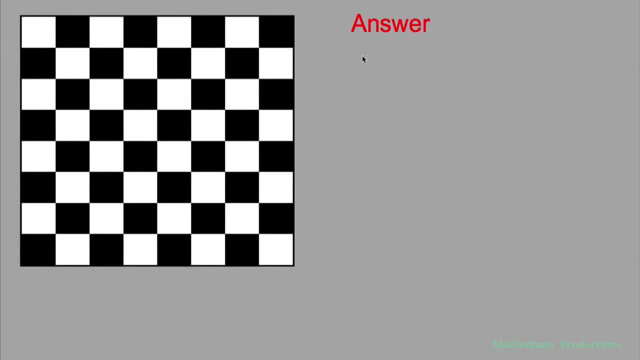 video and play it back when you're ready for an explanation. All right, let's go over this answer really quick. Let's start with the obvious. If you count individual squares, the little squares, there are 64.. I hope you didn't count one by one, because you could just count the row. 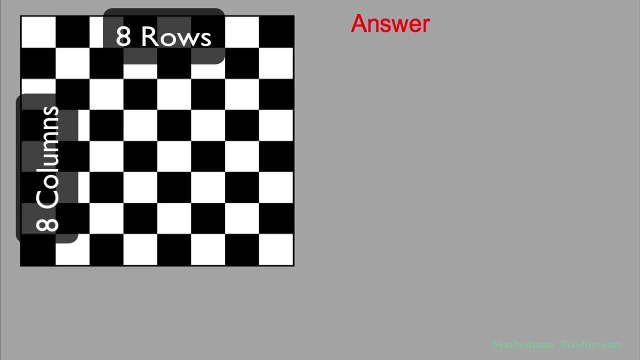 and the column and multiply them together Eight times eight, and we get 64.. But that's not all the squares that exist within this chessboard. If you take a look closer and you think out of the box, you can also make a square out of a two by two squares. For 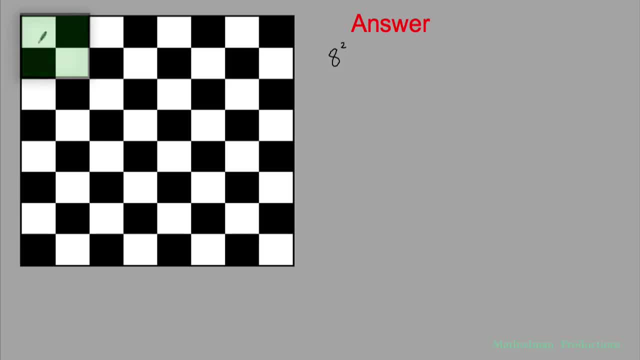 example right here, that's one Going through this first row. I can make seven of those: One, two, three, four, five, six, seven. At this point I can't make another two by two, so there's only. 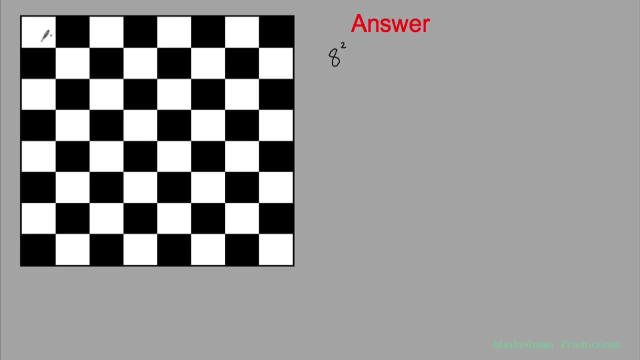 one square out of this row, And if I do the same pattern, there are seven in the first column: One, two, three, four, five, six, seven. Seven by seven is 49, so I can add seven squared to this count. 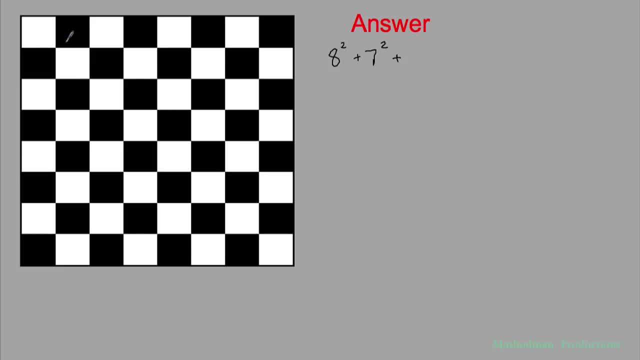 Now thinking out of the box again, instead of a two by two, I can do the same with a three by three. There is a three by three square that I can make out of this chessboard. That's one, two, three. 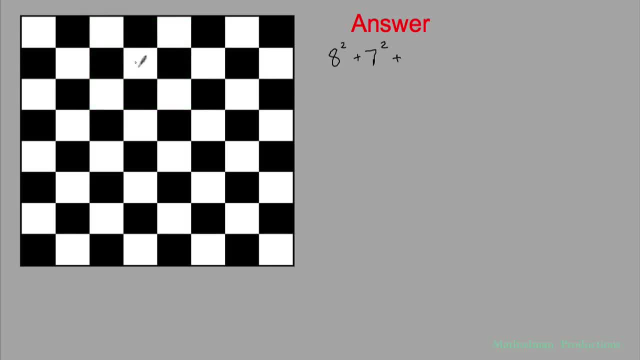 and if I keep going, I can make another two by three. And if I do the same pattern, I can make another two by three. And if I keep continuing that pattern, there's six of those three by three squares on the first row. Likewise, there are six three by three squares on the first column. 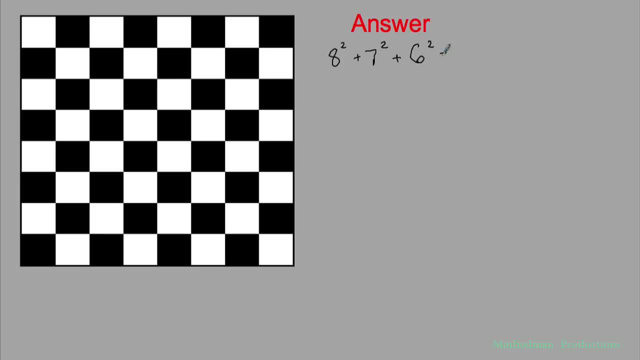 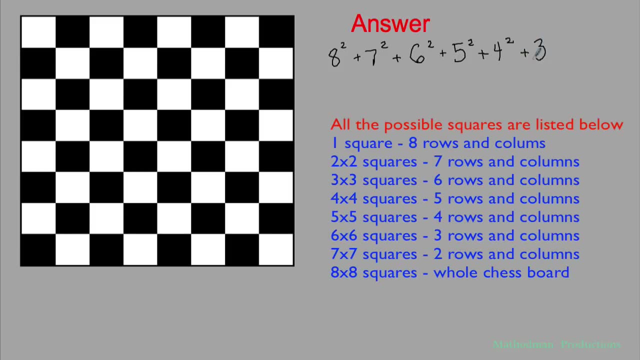 so I can add another six squared If I keep repeating the pattern. if you look at the pattern, it's eight squared seven squared, six squared. Each number is just going down by one and you're squaring that result. So if I were to continue this, I would get three squared. 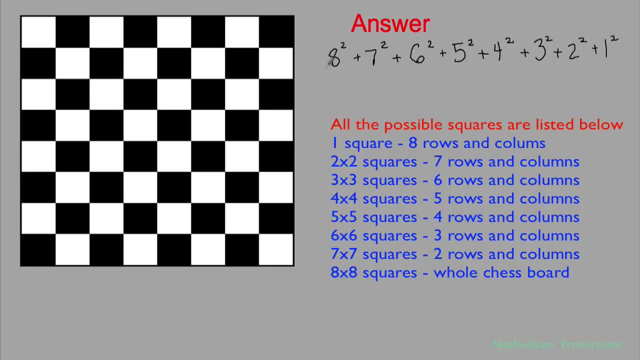 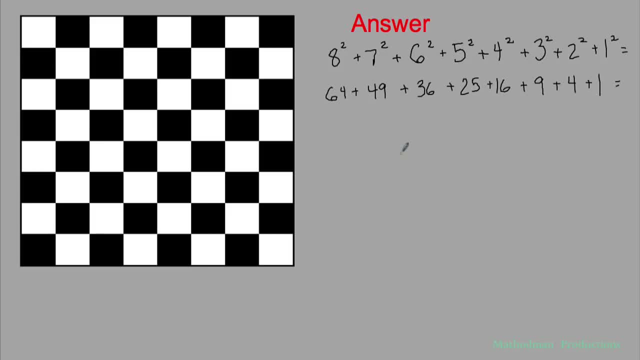 plus two squared plus one squared At the end. if you add all those up, that's the simplified version of it and the final answer is two oh four. Hope you like this puzzle and I will have more for you in the future, But for now, don't forget to subscribe to my channel, and I just